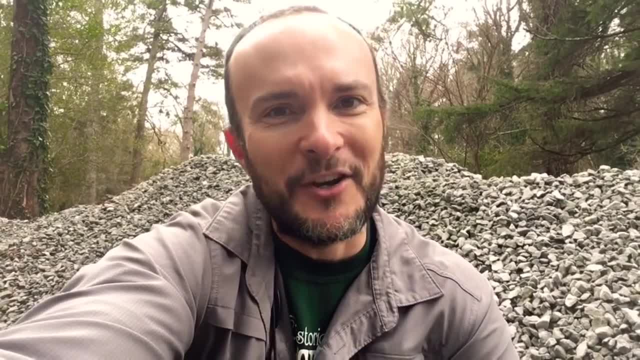 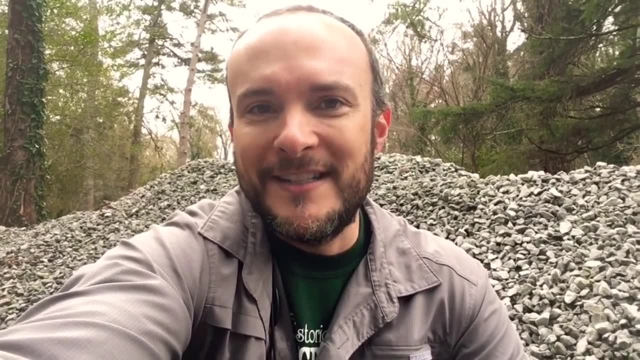 and you know what a pain it can be when your house shifts or when things aren't the way that you want them, or when it's got a permanent problem that you're never going to be able to fix it's designed in. that is way worse. So I know that Some of you know that. For those of you, 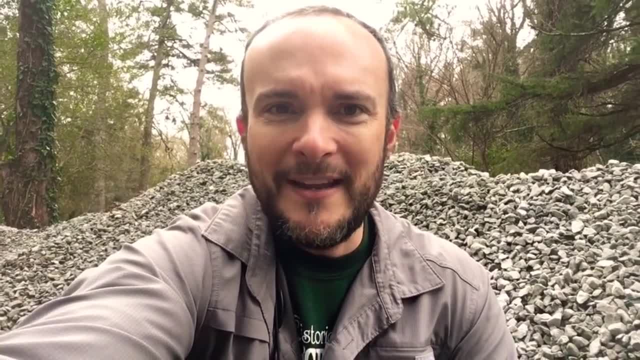 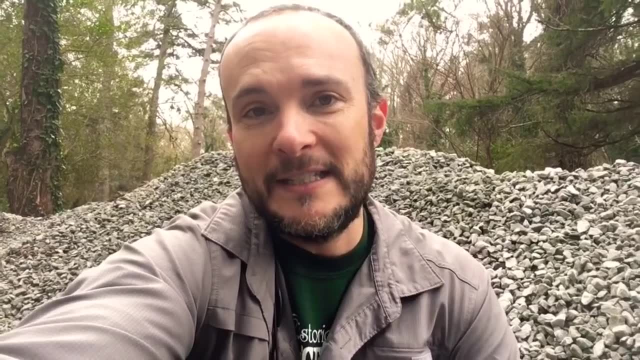 who don't, you will find out. So we're doing this the right way: The $1 fix versus the $10 remediation during construction versus the hundred times as expensive fix once we're done. So check out what's about to happen when you start digging into. 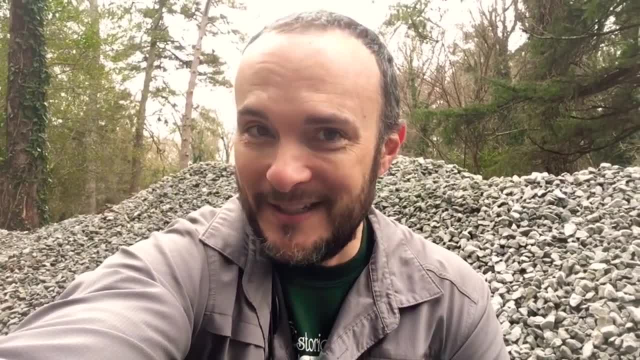 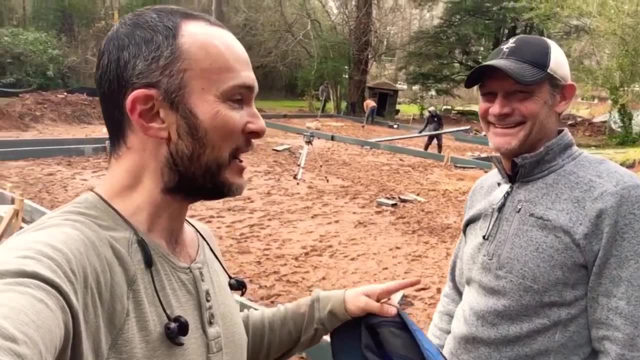 how high performance the pad that you're building your house on actually is Looking good, right, Yeah, All right, Got my brown shirt, Got my geotechnical engineer. It's more important. So Jeff is back and he's going to look at the state of our forms. So, because we 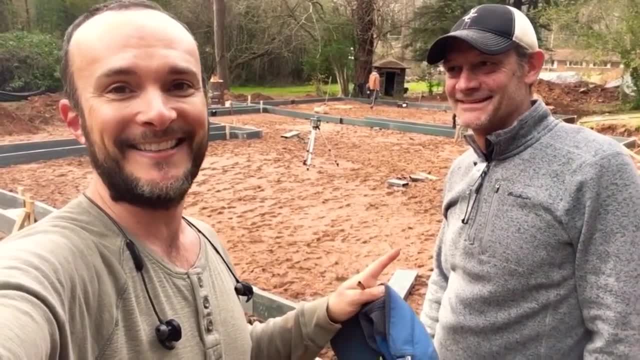 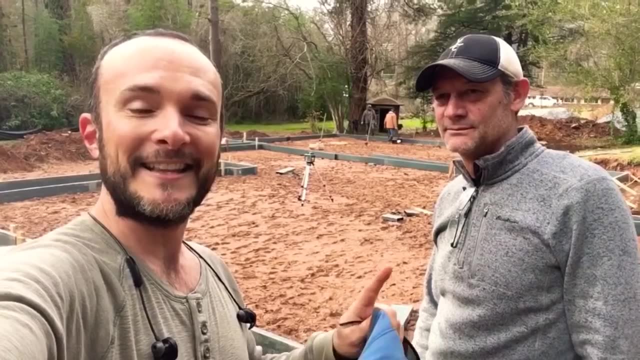 are about to pour concrete and this is the last minute when anything that is, on his report, which took a long time to compile and do all this stuff. for if we don't follow the directions at the last minute, here it's just a piece of paper, right, It's just like. what are we going to do? 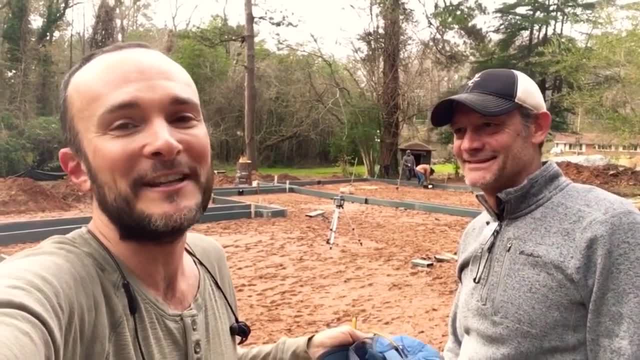 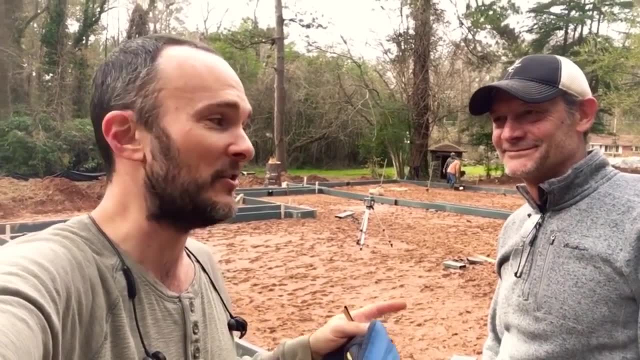 Like performance Essentially. Yeah, Like I could give you a heat load calculation. but if you're not actually going to build the house the way that we said, it doesn't matter what the design stuff is, It's like what actually happens on the day of. So that's why I got like this Comes out with: 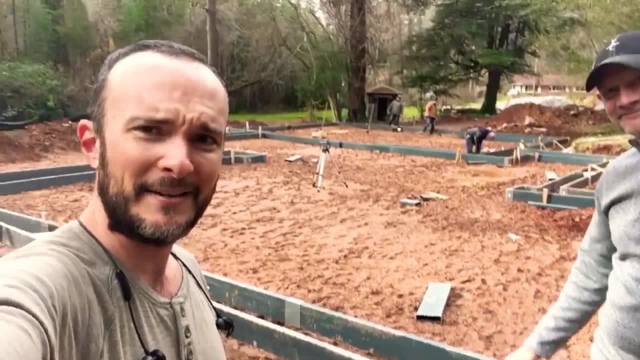 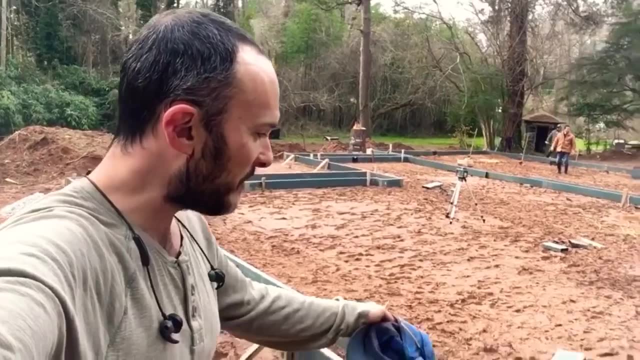 this high-tech tool. Show them your tool. High-tech, Yep, Okay, That was. you have to buy that from an engineering store. They have an engineering bookstore for all engineers, Okay, So show us what we're doing here. Well, essentially, Corbin did do things the right way, Placed a lot of fill. 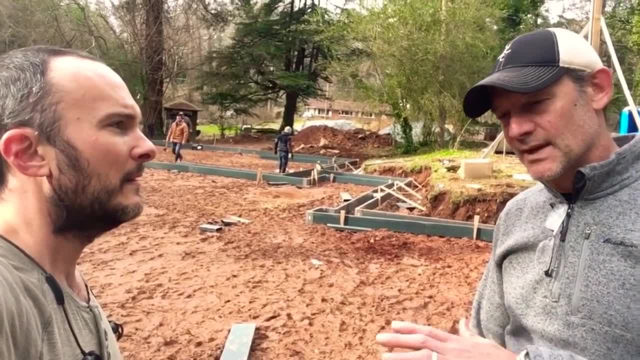 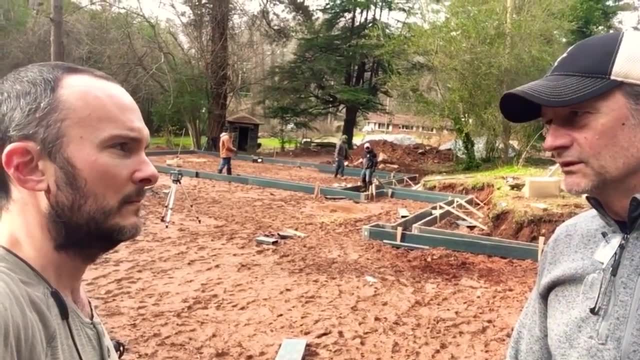 in here and we talked through the whole process when he was building the house. So that's what we're putting it in. So he's compacted it in layers and everything was great. But it's like having a recipe to bake a cake: If you got the perfect recipe but you eliminate some ingredients. 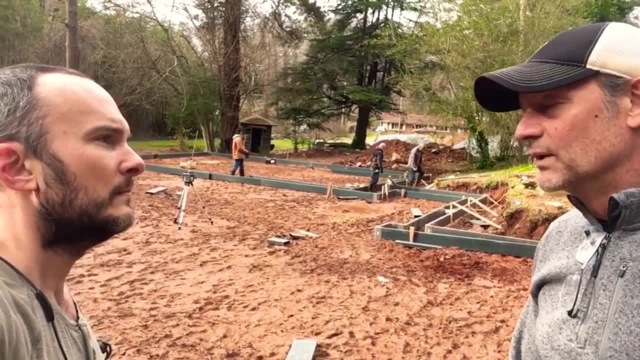 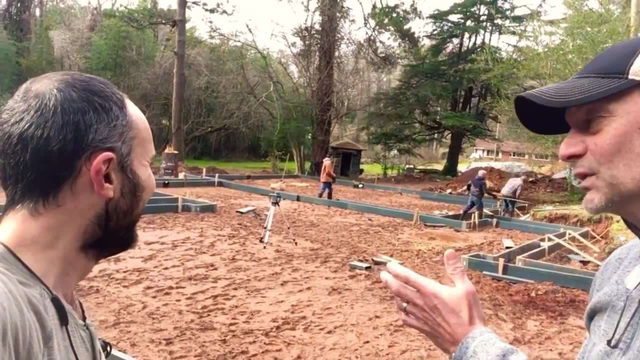 you'd have a problem. So similar thing here. Things were done, but that's been a few weeks. We've had some weather conditions, Which happens. that weather It does happen, It happens regularly. So before we actually put concrete and cover this up so that we can't deal with it later, 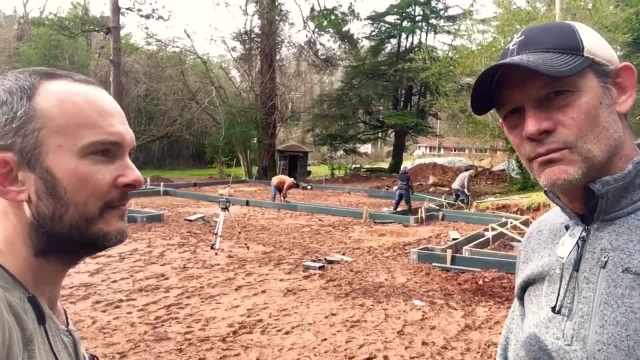 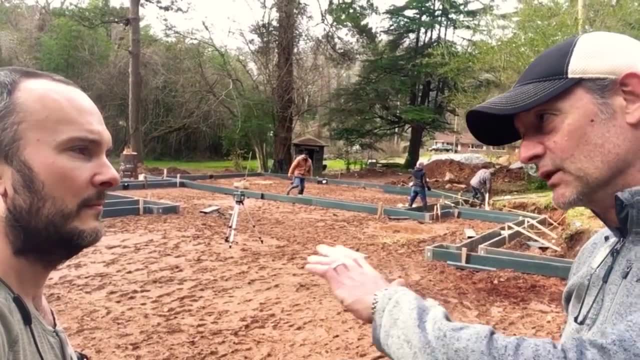 we're going to take one last minute, look at the soils at bearing level beneath what will be the foundations, and just make sure that we're doing the right thing. So we're going to take a look at what we put in so diligently, or that you put in so diligently is representative of what the 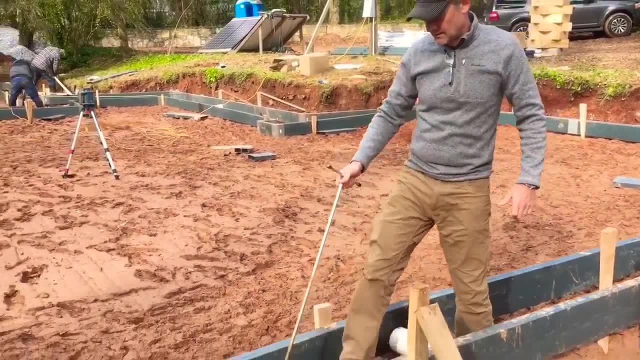 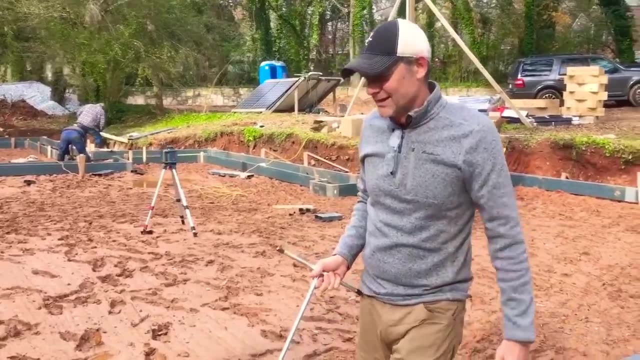 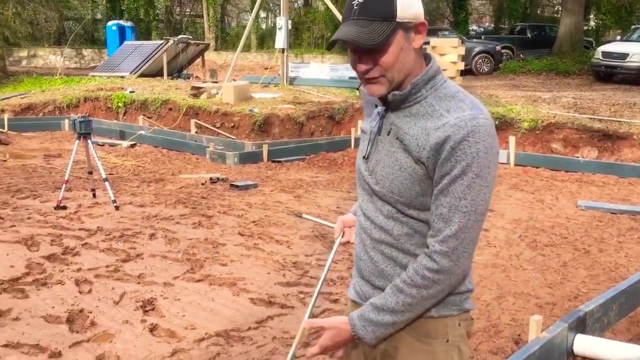 home's going to actually sit on. So that's what we're going to do right now. Awesome, Very technical procedure. Yeah, How many PSI are you putting on that? Well, I'm not a heavy guy, but this is a pretty sharp point. So the pressure is decent Now back here. it was dry. 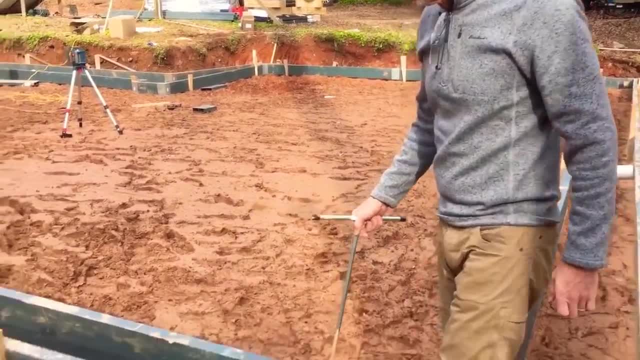 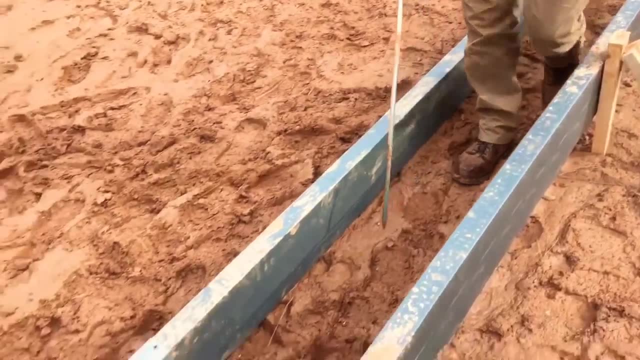 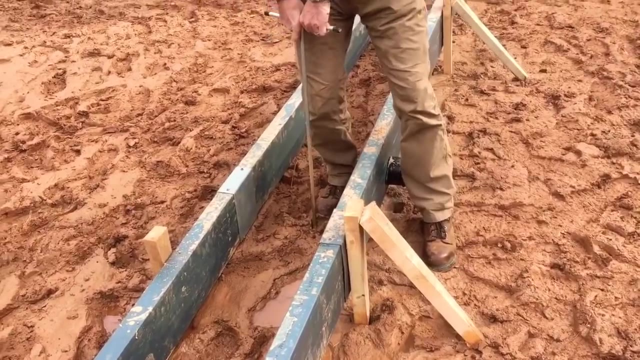 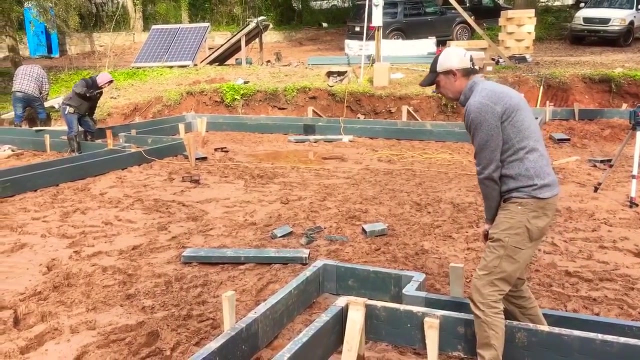 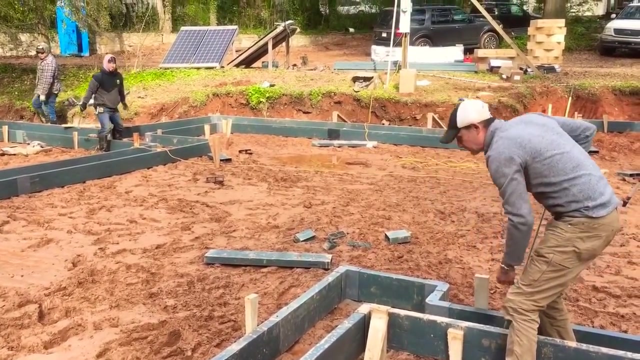 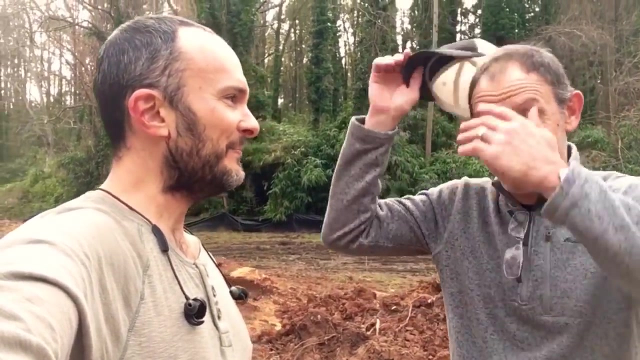 Over there specifically, it didn't get wet at all because we tarped over this whole thing. Okay, Take my hat off again, because this time it's for bad news. Do I need mine off? You don't need to take yours off, You're the consultant, Mine's off. Yeah, Your job is to tell the truth all the time. 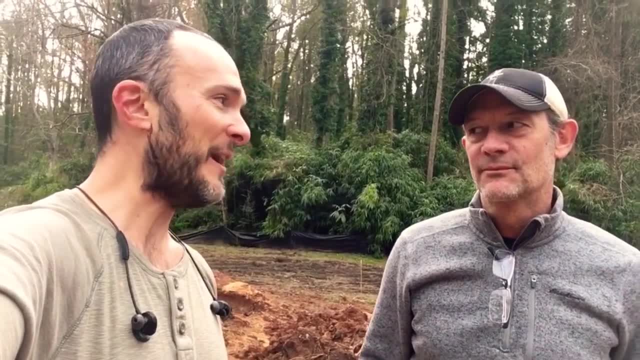 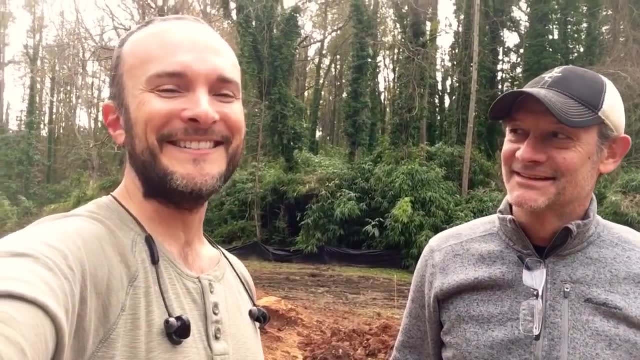 So the reason you bring in a third part of air fire is because- and Jeff offered this morning like hey, do you want me to come out there and look? And I was like part of me thought I don't want to know, But part of me said 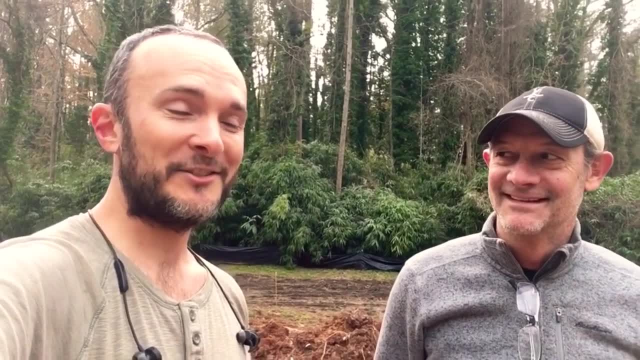 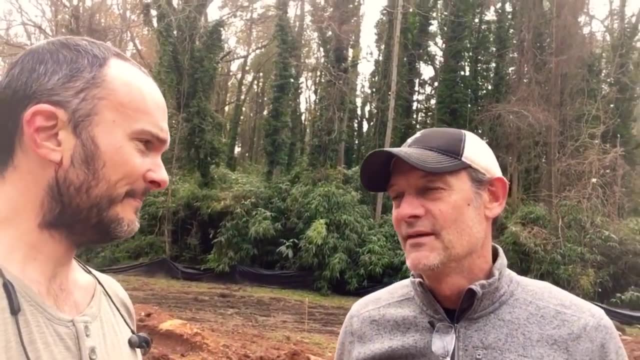 this is a construction site, Just to remind everyone that having a third party come out and look at it is important. And what we found is what? Well, we found some soft soils directly beneath where the footings are going to be constructed. So the material was put in and 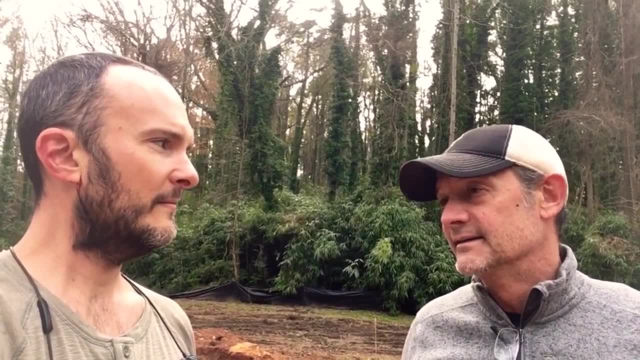 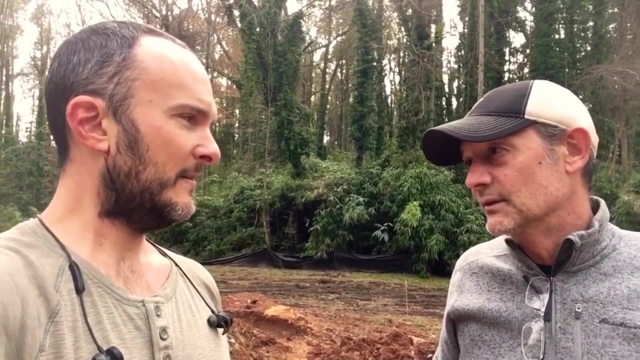 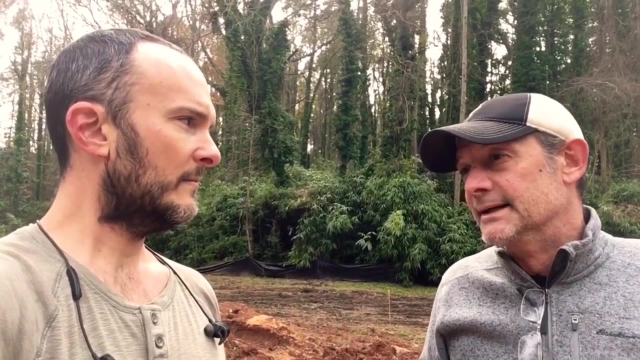 compacted well, but we've had the weather that we talked about and some activity with equipment and people just walking around that has softened the upper eight to 12 inches of soil directly beneath the footing Or where the footing will go, And that material's pretty soft and compressible And so, to be honest, 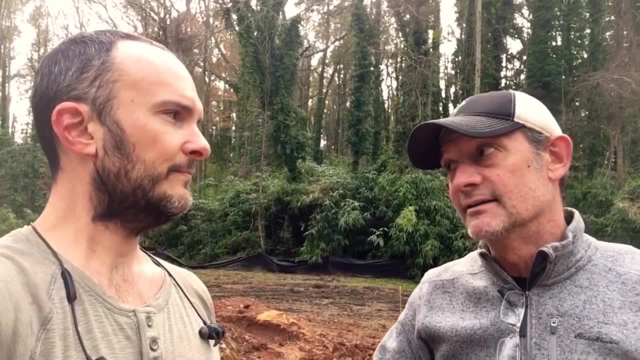 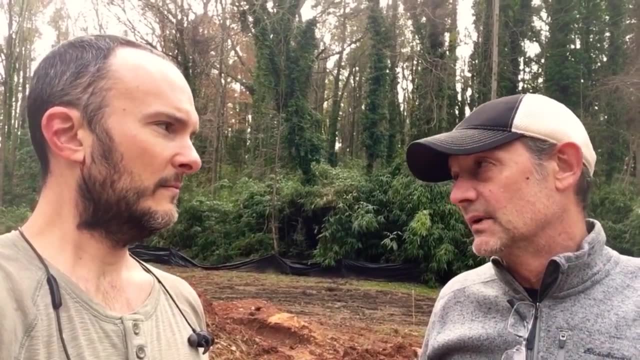 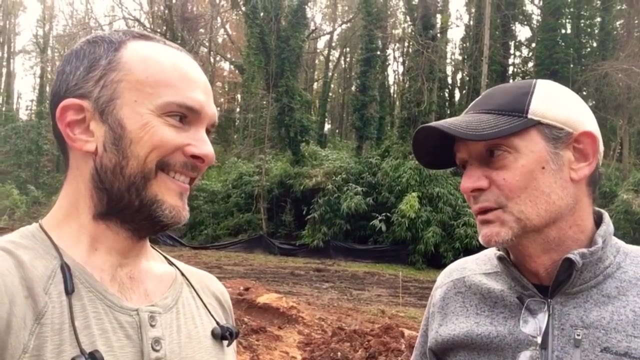 before you get concrete into the trench, and that's your footing and it's covered and done. it's so much easier and cost effective to just reduce that risk by taking out the very soft soils and replacing it with something else like stone or something fairly incompressible. 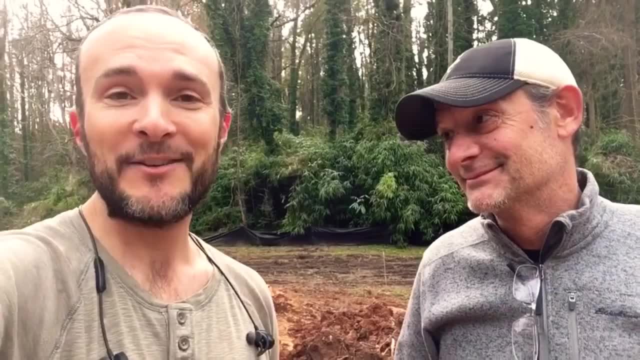 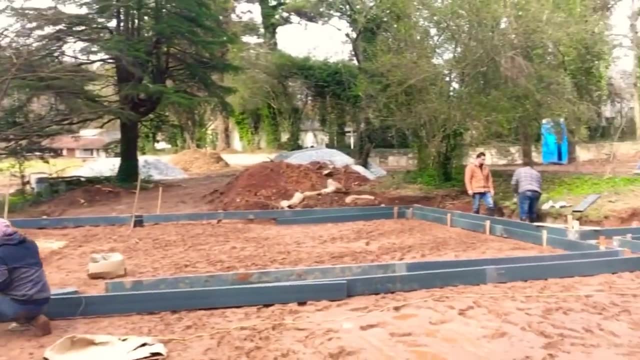 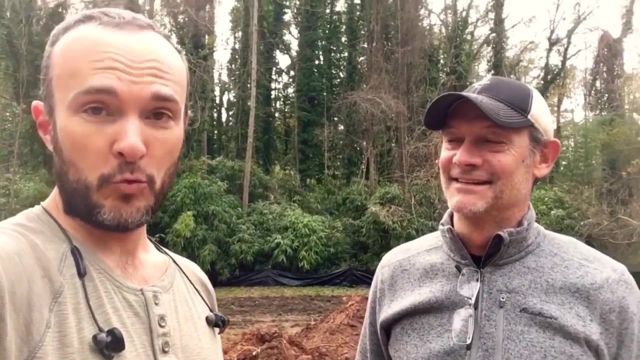 Right. So that's engineer speak for the top eight to 12 inches is bad. We need to take it out with a shovel, So we're just going to go around the entire strip footing. I've got my help here and we're going to do this on a nice dry day. Take out the soil, put down the rocks.